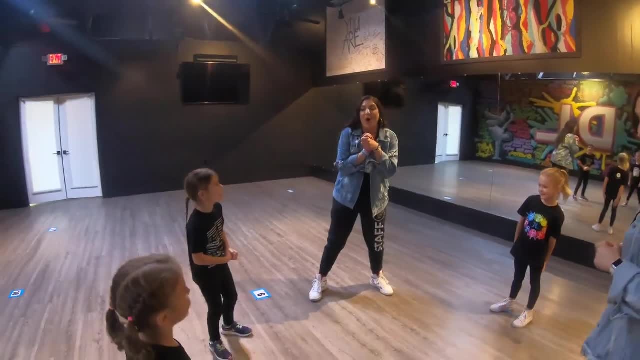 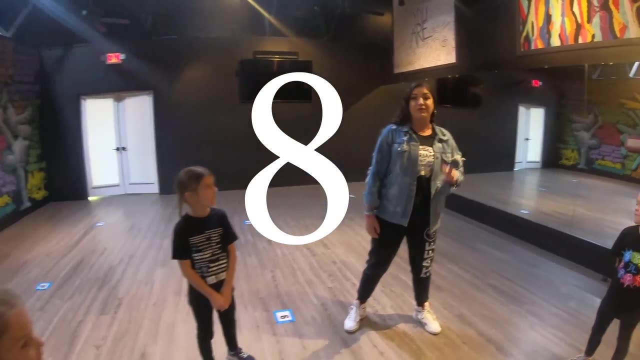 All right, girls, are we ready to have fun today? Yeah, Okay. so let's remind everybody: What number do we count to in dance Eight? Very good, And we have two types of hands in hip-hop. What are these? 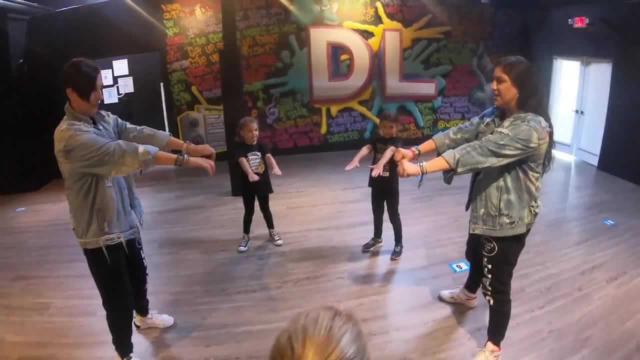 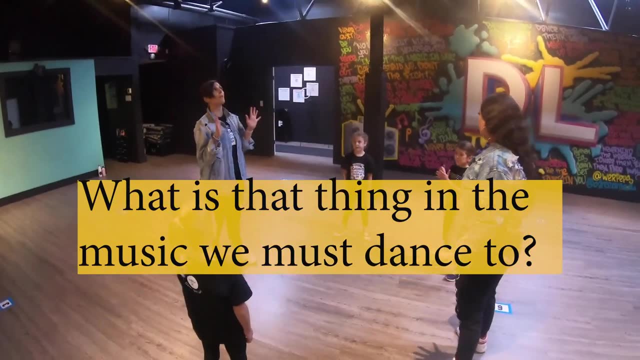 Good. And what are these? Excellent, Let's do it together Ready. Fist leg, fist leg. Let's go really fast. Fist leg, fist leg. Very good, All right, And what is that dance music that we must dance to? Eight, What dance? The beat. The beat, Yes, very good. 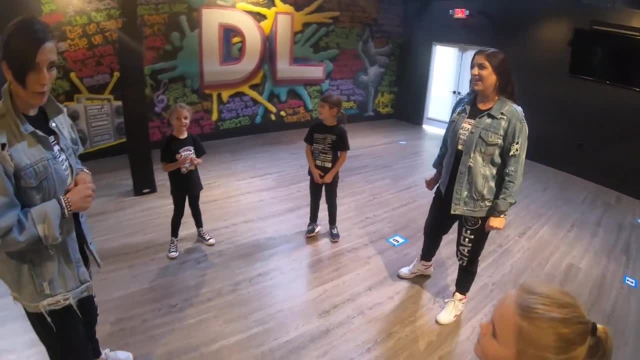 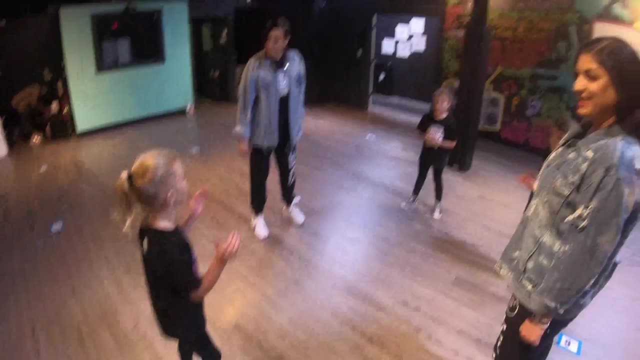 It's okay. So are we ready to find the beat in our bodies? Yes, Okay, Charlotte, you ready. All right, let's go to hip-hop. Five, six, seven, eight. One, two, three, four, Five, Six, seven, eight. 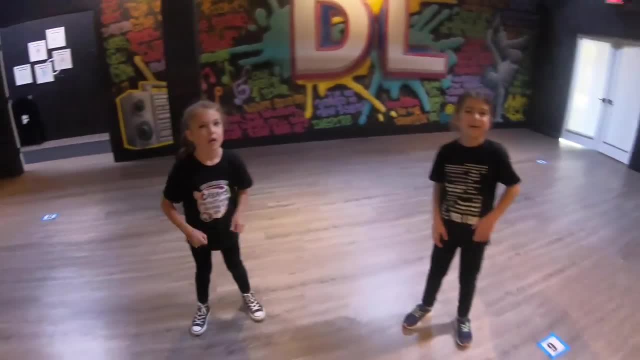 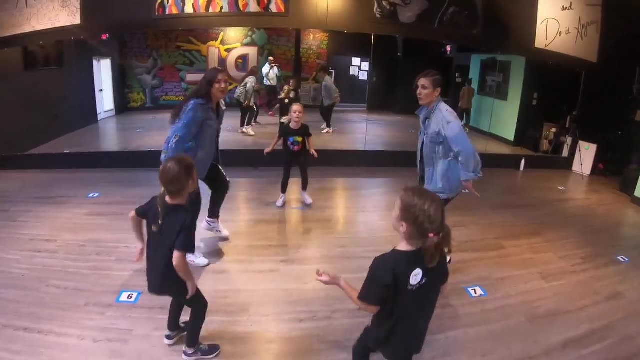 One, two, three, four, Five, six, seven, eight. One, two, three, four, Five, six everybody. One, two, three, four, five, six, seven, eight, Five, five, six, seven, eight. 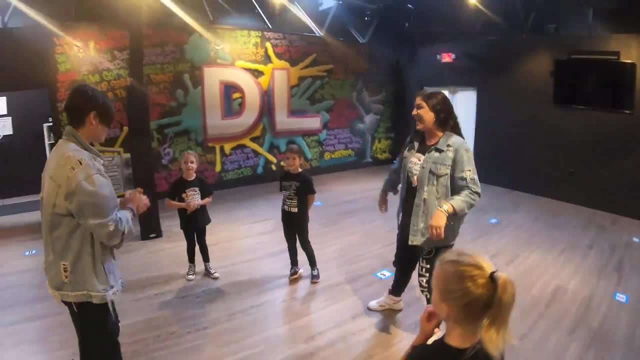 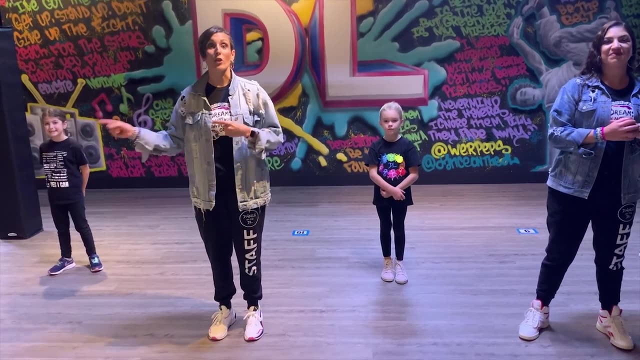 Are we ready to dance? Yes, Good, good, Do it girls. All right, girls. are we ready to learn our dance? Yes, Okay, we're gonna start with step together, step touch going to the right side, so our right foot is going to. 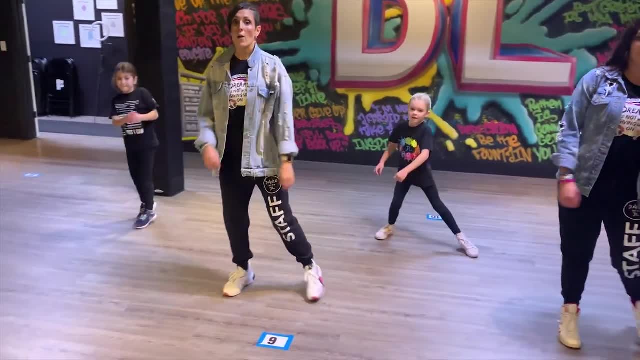 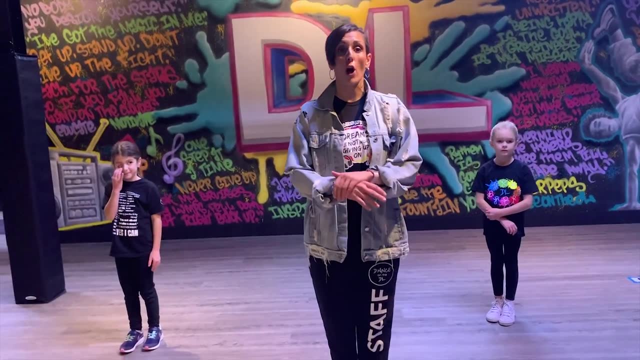 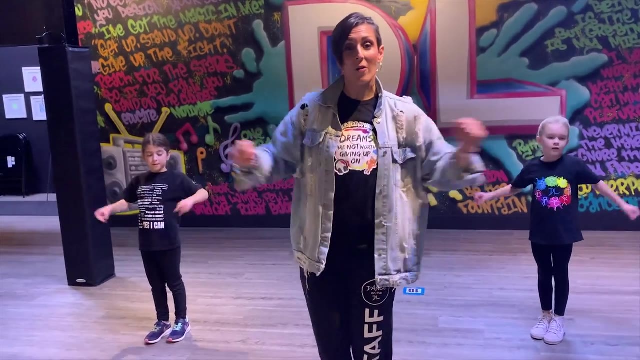 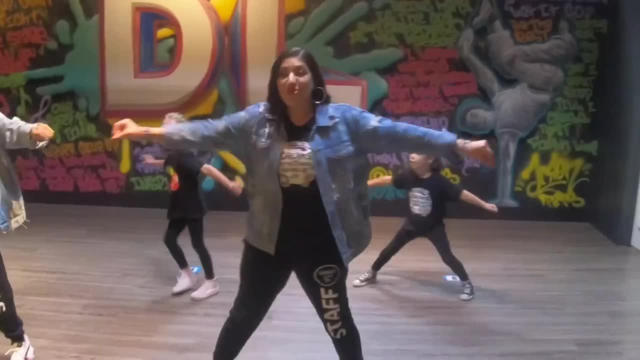 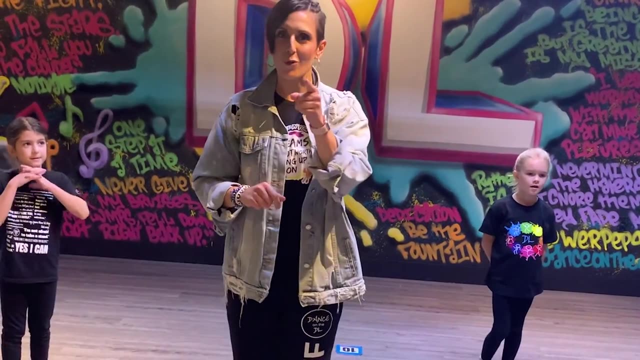 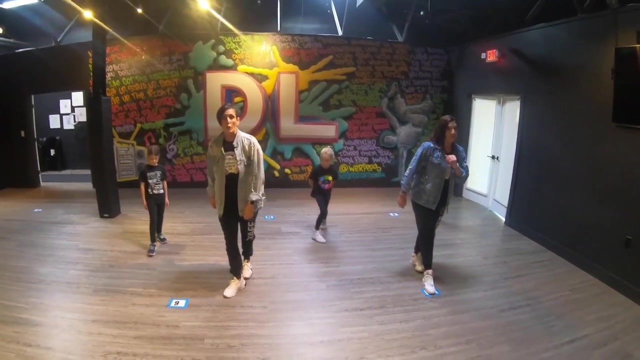 seven. here we go: one, two, three, four, five, six, seven, eight. amazing job. you guys are doing great at home too, I can tell. let's start now with a box step. so we're gonna stick our right foot forward, that's one. we're gonna cross our left. 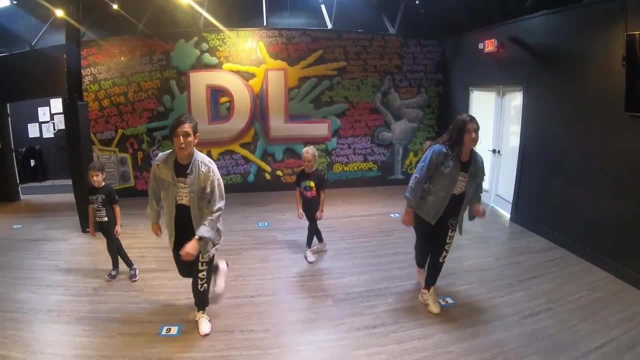 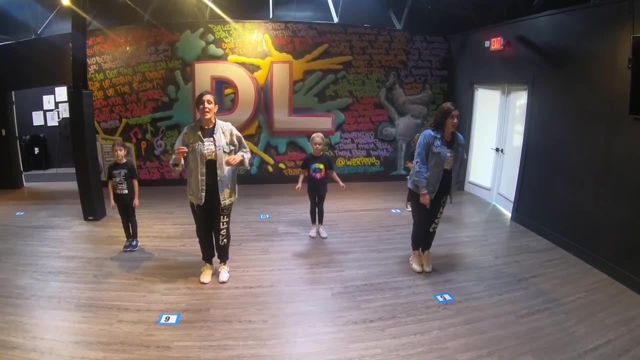 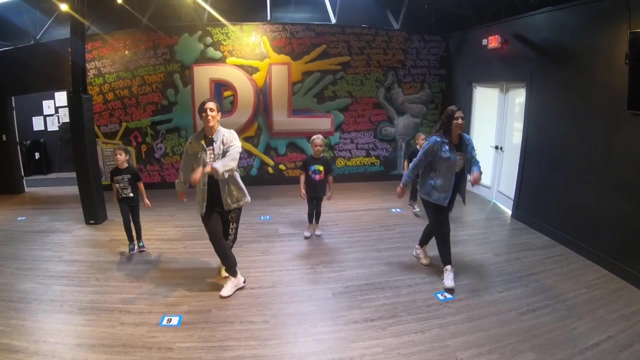 foot over our right. two: you're gonna take your right foot back. three: bring your feet together. four: amazing job. let's try that again. in five, six, seven, eight we go one, two, three, four, five, six, seven, eight, cross two back together. four: one more time: here we go: one, cross, two back. 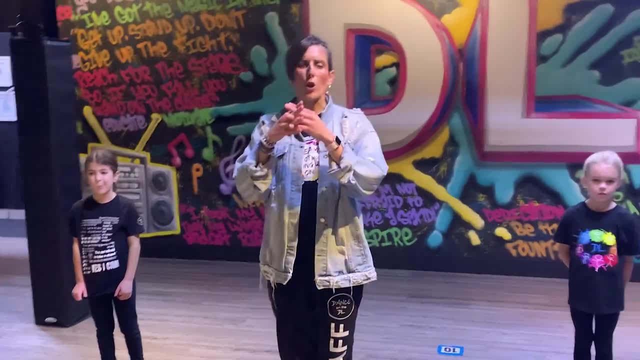 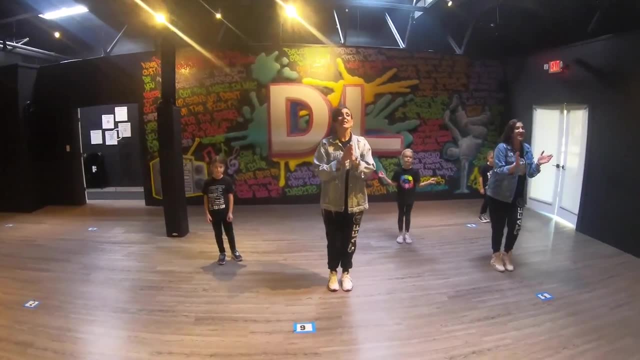 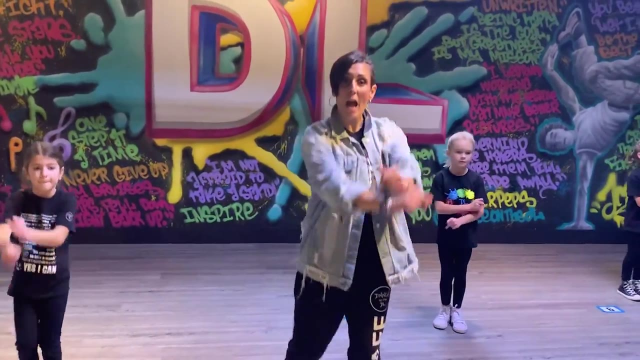 together four. good job. okay, now let's just put those two together and then we'll add on our last two steps. does that sound good to everybody? yes, here we go ready in five, six, seven. here we go over one, two, three, take it back five, six, box. step down, go one, two, three. last time five, six, seven. 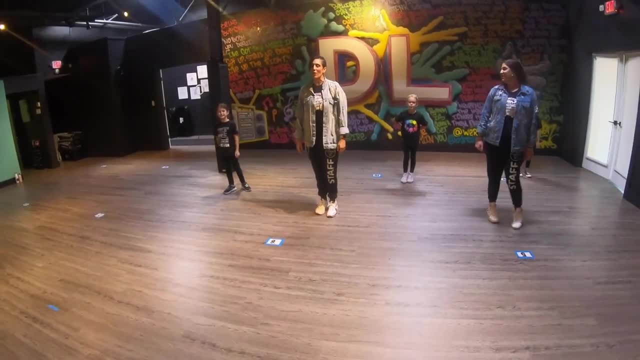 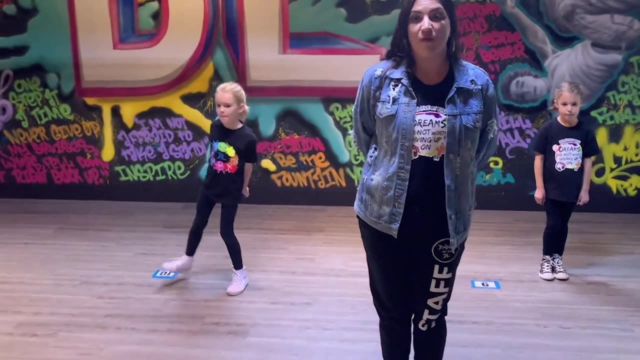 eight: amazing, great job, baby, very cool. next we're gonna do the smurf- so much fun. so the first we're gonna start with our feet, so we're gonna take a step over, we're gonna go and one and you're gonna bounce two, two, step the other way and 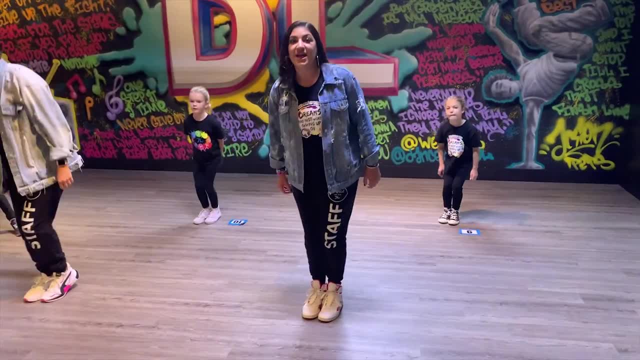 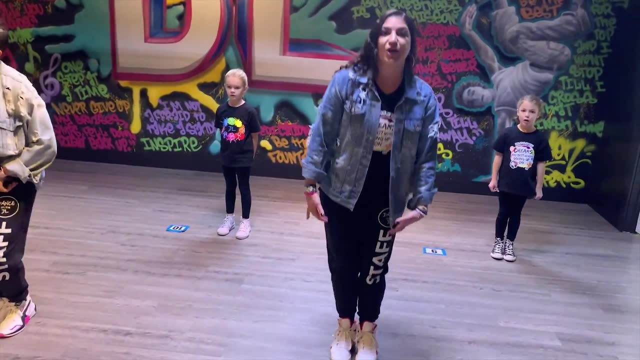 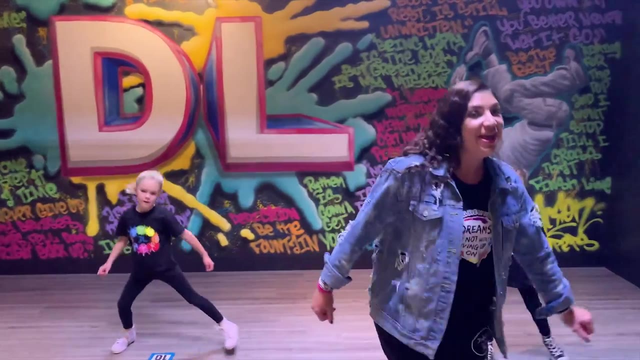 three, four and five, six and seven, eight. don't forget to bounce those knees, girls, because it's hip hop, we gotta bounce. good, all right, let's try the feet one more time: five, six, seven, eight and one, two and three, four and five, six and seven, eight. very good, that looks. 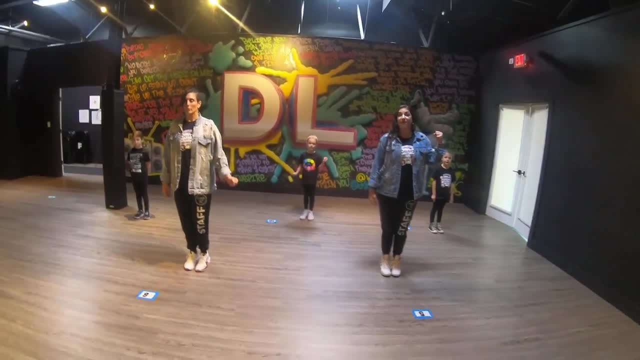 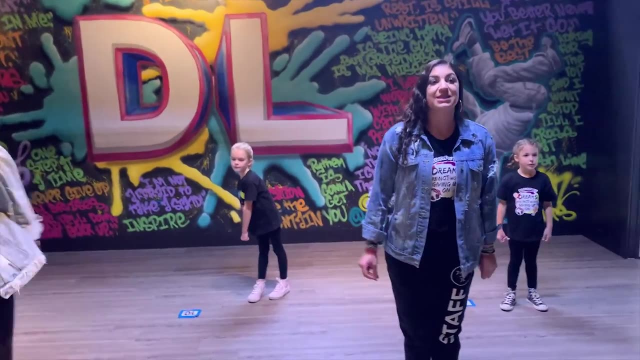 super cool. but we're gonna add a little arm, so we're gonna take our hand in that fist that we learned and we're gonna put it in our pocket across our body. very good, so let's try it with the hands. five, six, seven, eight and one, two and three. 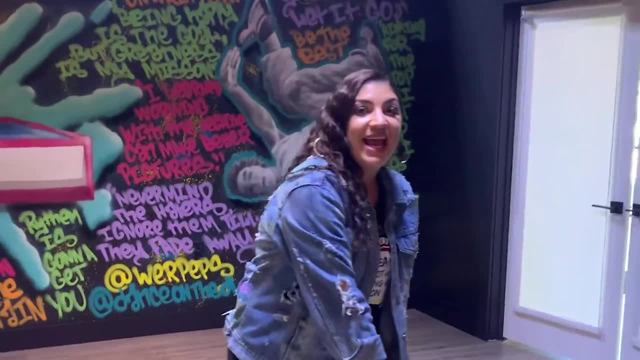 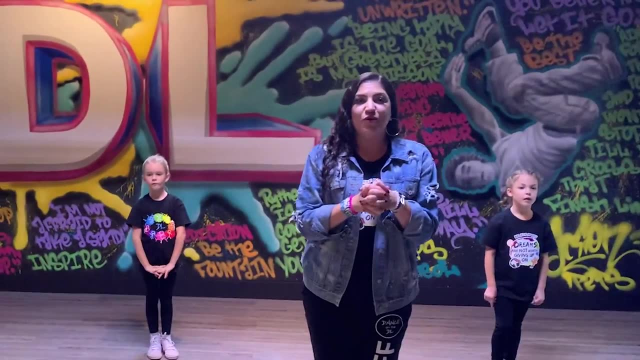 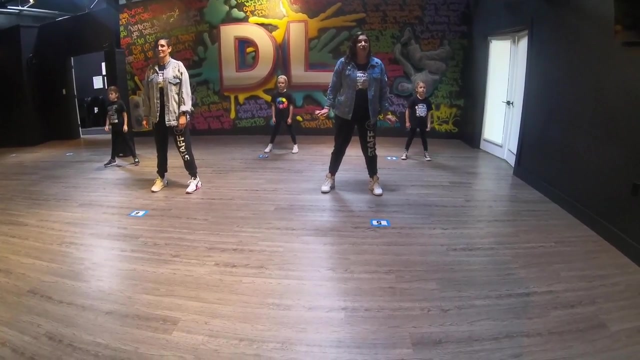 four and five, six and seven, eight, excellent, okay, last move, and then we'll glue it all together. so our last move- another fun name: it's called the bismarck key. so we're gonna take our feet apart to start and we're gonna do a tiny little jump not too far off the ground. we're gonna jump one, then we're gonna swing our. 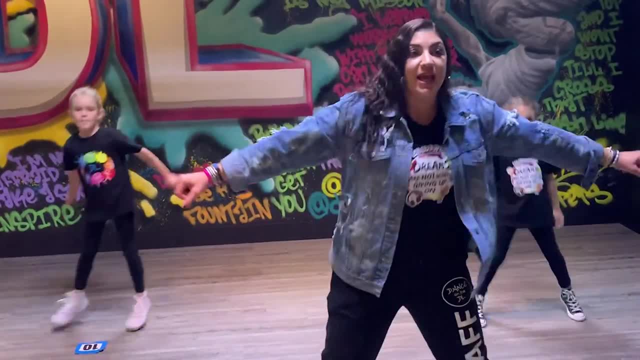 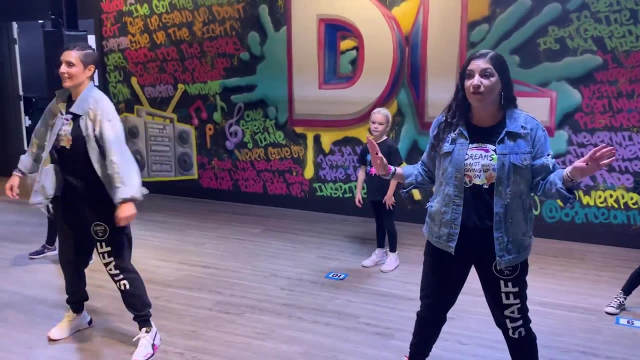 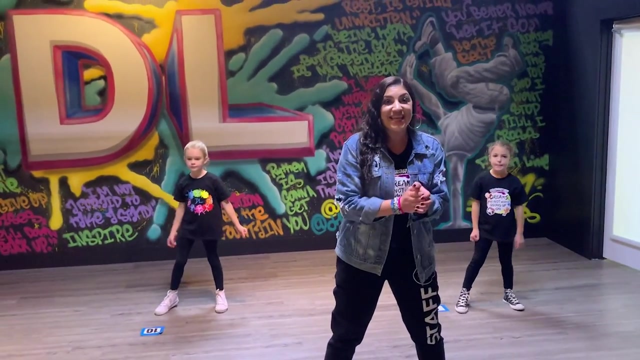 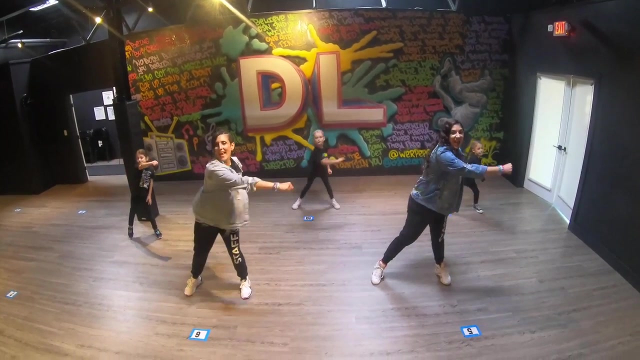 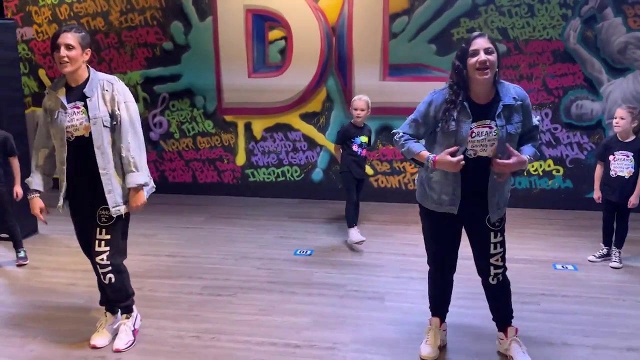 arm in front of us. two, jump again. three, swing that other arm. four good, five, six, seven, eight. very good, we're gonna take that a little faster. don't forget to bend our what knees. very good, all right, let's try that again. five, six, seven, eight. we go one, two, three, four. five, six, seven, eight. awesome. okay, let's take it all together from the top. very good, very good, all right. time to sing this, Linda, all right?